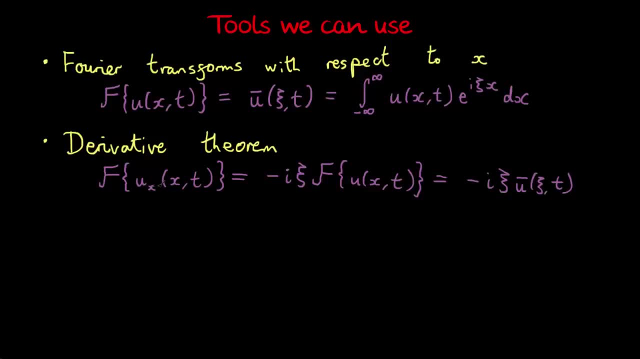 take the Fourier transform of a derivative- in this case the derivative with respect to x, because we're taking the Fourier transforms with respect to x- then that is exactly the same as minus i xi times the Fourier transform of u, or in other words, minus i xi times u bar. So that's the derivative theorem We've. 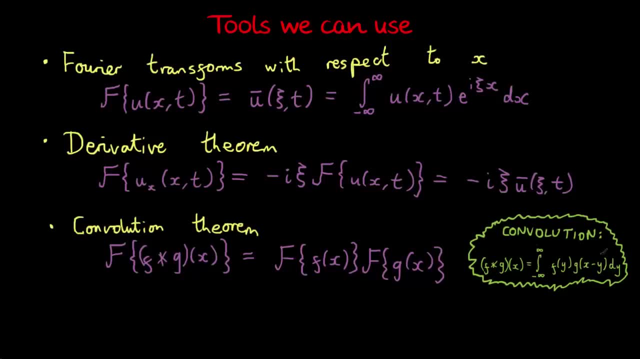 also got the convolution theorem. Here's the definition of convolution in green. But the convolution theorem says that if you take the Fourier transform of a convolution then it's exactly the same as the product of the two Fourier transforms. So the Fourier transform of F, convolution g, is equal to the Fourier. 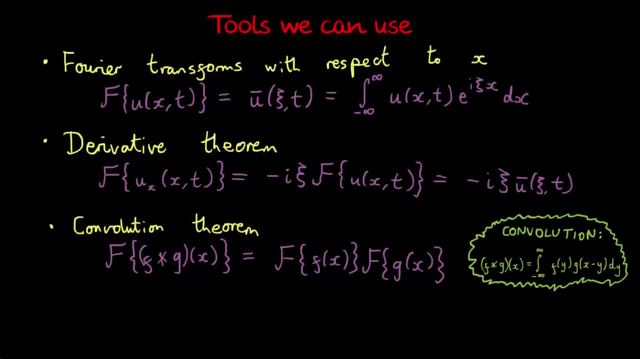 transform of F times the Fourier transform of g. And then finally in our toolbox we've got the Fourier inversion theorem and that tells us how to get the function u of x and t back if we're working from the Fourier transform. So if we're 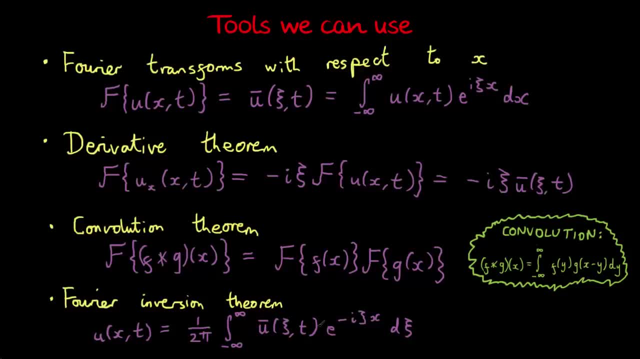 we've got the Fourier transform u-bar of xi and t And the Fourier inversion theorem says that the way that we do that is: we take u-bar of xi and t, we multiply by e to the minus i, xi, x, and then we integrate with respect to xi. 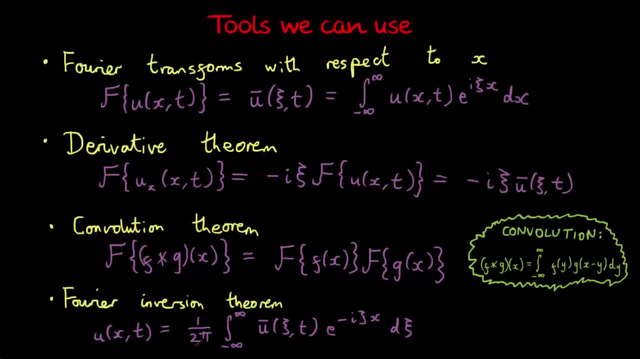 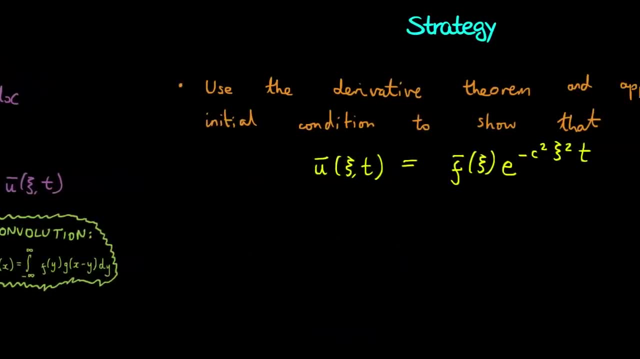 between minus infinity and infinity, and then multiply by 1 over 2 pi. Okay, so those are the tools that we're going to use. What about our general overall strategy for solving the heat equation? Well, first of all, we're going to use the derivative theorem. 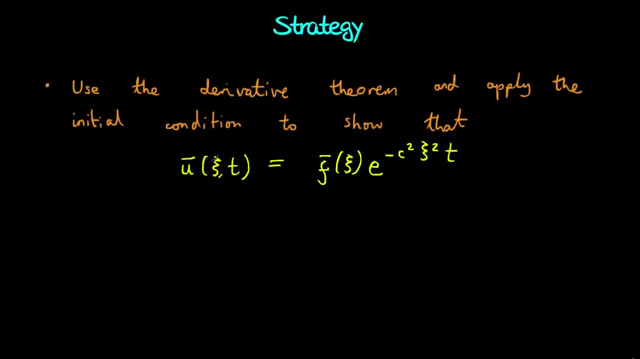 and apply the initial condition, and that's going to allow us to show that u-bar, the Fourier transform of u, is given by this expression. here, f-bar times e to the minus c, squared xi, squared t. So, in other words, we first of all find an expression. 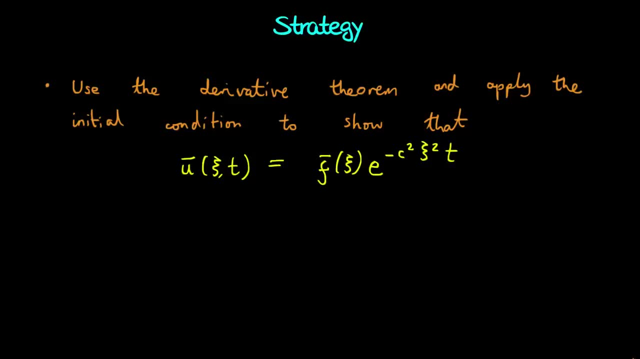 for the Fourier transform of u And we're going to use that expression for the Fourier transform of u. Then the second step really is all about inverting the Fourier transform. So we've got an expression for u-bar. How do we get back to u? 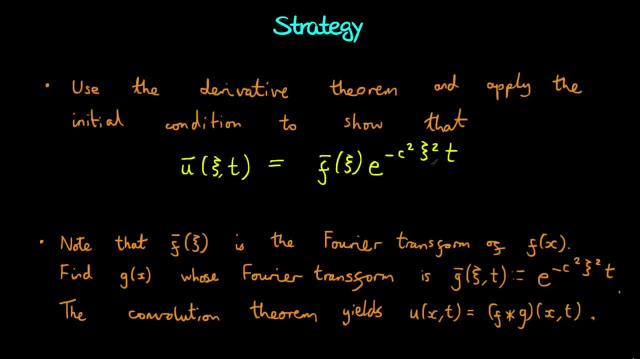 Well, if we look at the right-hand side of this expression in yellow, then we can say that the Fourier transform f-bar is just the Fourier transform of f. So we know what the inverse Fourier transform of f-bar is. But what about this other function here? 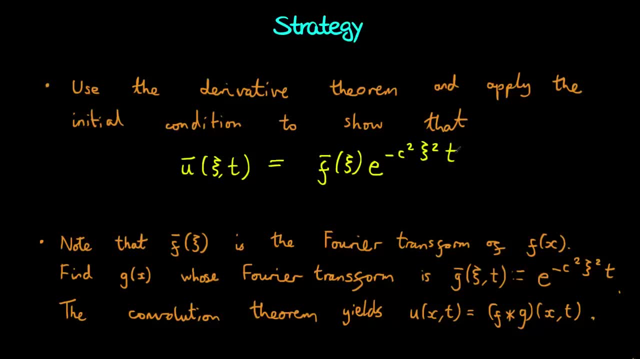 What about e to the minus c, squared xi, squared t? Well, we're going to call that g-bar, just to give it a name, And then we're going to try and find its inverse, Fourier transform, And that's going to be where the Fourier inversion theorem comes in. 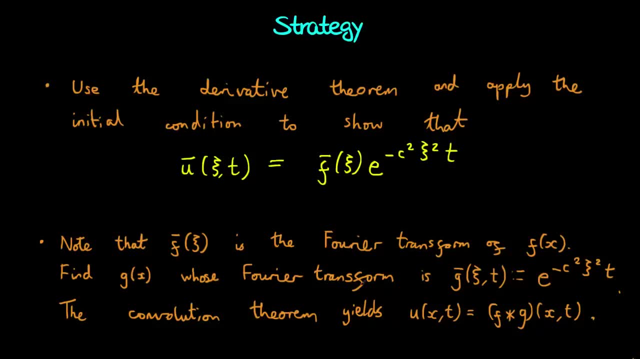 That's going to allow us to find the function g, whose Fourier transform is g-bar, And then, finally, we'll say that: well, we have that u-bar is the product of Fourier transforms. Well, the product of Fourier transforms. we can use the convolution theorem to 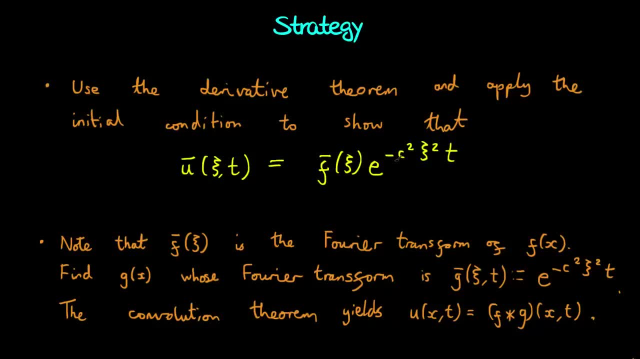 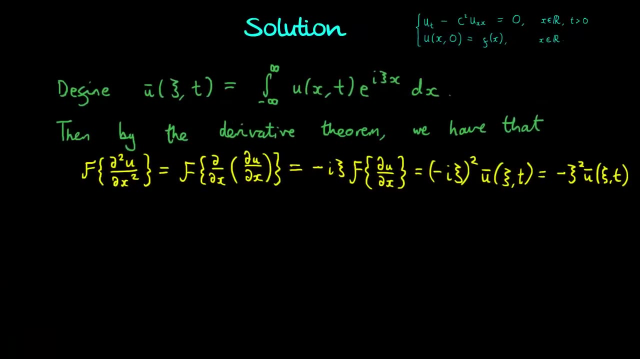 to write as the Fourier transform of the convolution, And therefore u will be a convolution of f and g, And that will finish the derivation. Okay, so that's an overview of the strategy we're going to use. Let's start looking at it in a little bit more detail. 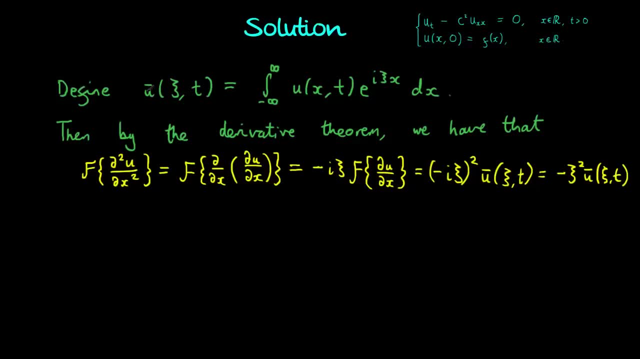 So first of all we should define what notation we're using. So we should say when we start writing the solution: define u-bar in this way here. So that's the Fourier transforms with respect to u-bar. So that's the Fourier transforms with respect to u-bar. 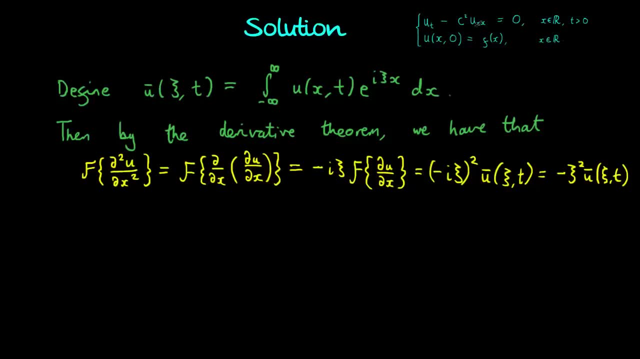 And then we're going to apply Fourier transforms to both sides of the heat equation. So when we look at the term uxx in the heat equation, we're going to use the derivative theorem straight away, Because the Fourier transform of the second derivative of u with respect to x. 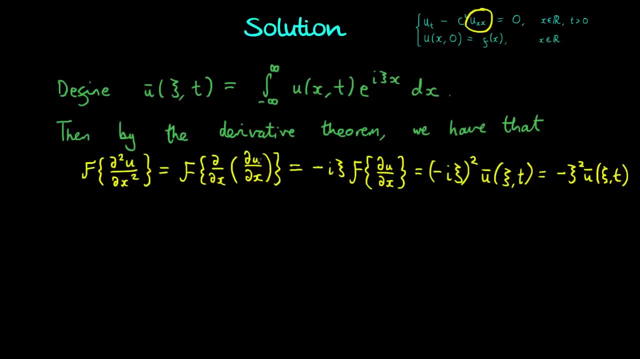 well, we can write that as the Fourier transform of the derivative with respect to x of du by dx, And then remember that the derivative theorem says that if we have the Fourier transform of the derivative with respect to x, if we have the Fourier transform of the derivative of something, 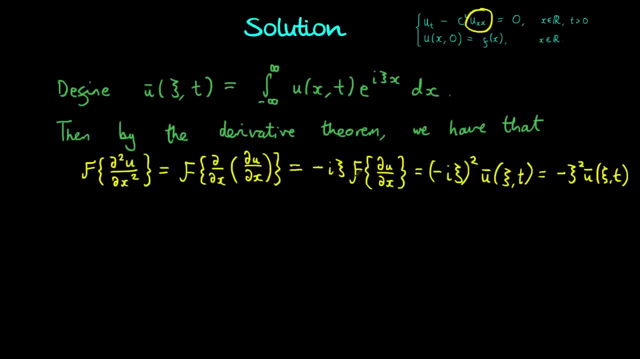 then that is exactly the same as minus i xi times the Fourier transform of that thing, in this case du by dx. Then we can say du by dx is a derivative itself, And so we can use the derivative theorem again. That means that we bring out another factor of minus i xi. 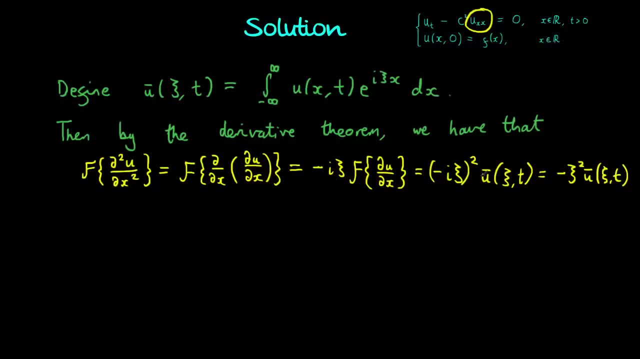 and then we'll have the Fourier transform of u, or in other words u-bar of xi and t, And then finally notice that minus i, xi, all squared will give us i squared, xi squared. i squared is minus 1, so this is just minus xi squared times u bar. 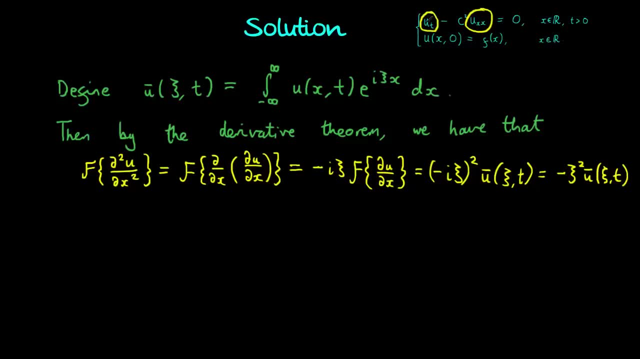 Now let's have a look at the other term in the heat equation. so u t. So if we want to take Fourier transforms of that with respect to x, then the Fourier transform of du by dt is just going to be du bar by dt. 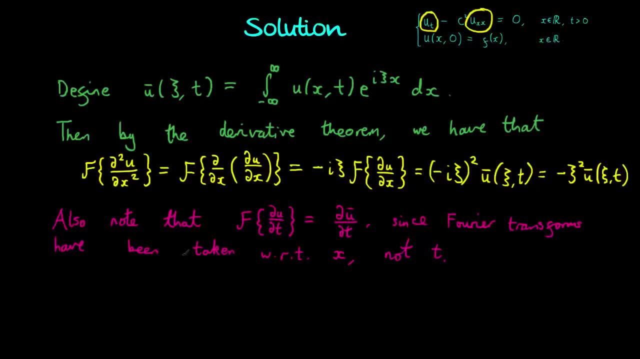 We're not going to use the derivative theorem here, because Fourier transforms have been taken with respect to x, not with respect to t, and so the derivative theorem isn't applicable if we're looking at derivatives with respect to t, So that's nice and simple. 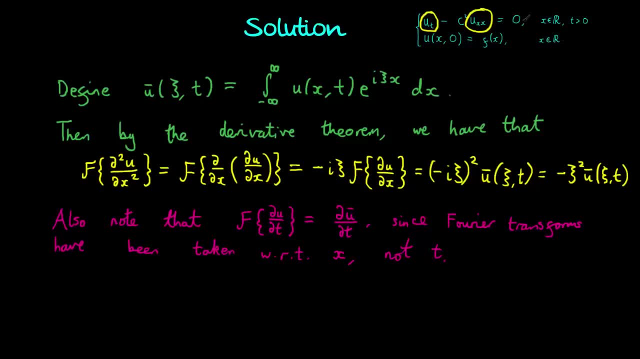 And finally, we should note that the Fourier transform of 0, which is on the right hand side of the heat equation, Fourier transform of 0, is just 0. You can see that very straightforwardly from the definition of Fourier transform. 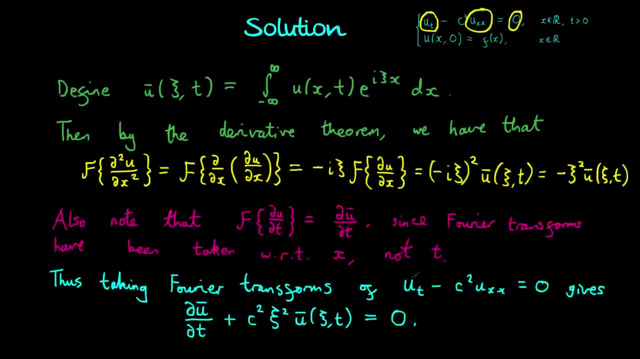 And so, combining all of that, if we take Fourier transforms of the whole of the heat equation of u t minus c, squared u x x equals 0, then it gives this equation at the bottom here. So the Fourier transform of u t we said was: 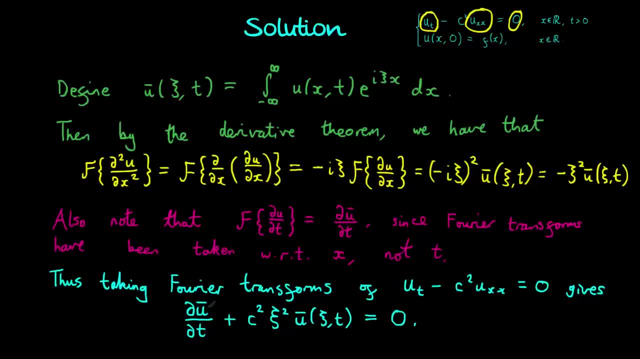 the derivative with respect to t of u bar. remember, u bar is a function of xi and t. and then we've got minus c squared times, the Fourier transform of uxx. so that's going to be minus c squared times minus xi squared, giving us plus c squared xi squared times u bar of xi and t. 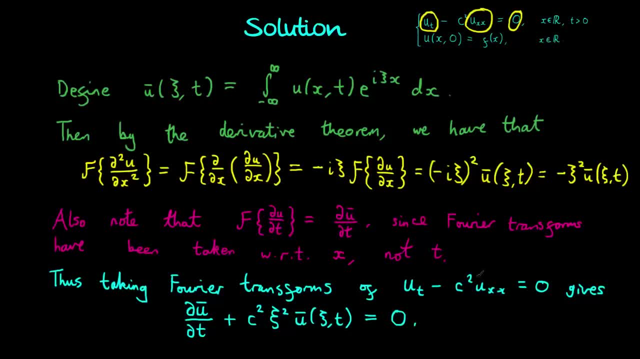 equals zero. so that is now something that looks a lot more like an ordinary differential equation, because we started off with derivatives with respect to t and x. now we only have derivatives with respect to t, and that's where the derivative theorem is so useful, because it's just allowed us. 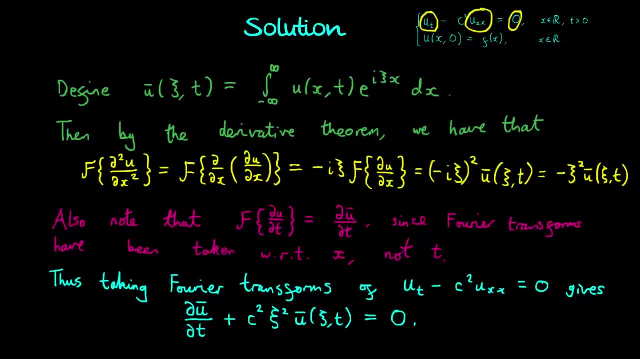 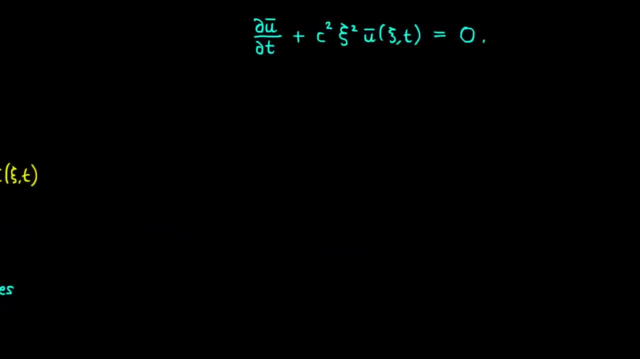 to essentially turn a PDE into an ODE, and that should be easier to solve. Having said that, let's see if we can actually solve it. So here is the ODE again. It's not quite an ODE because really u is a function of two variables. 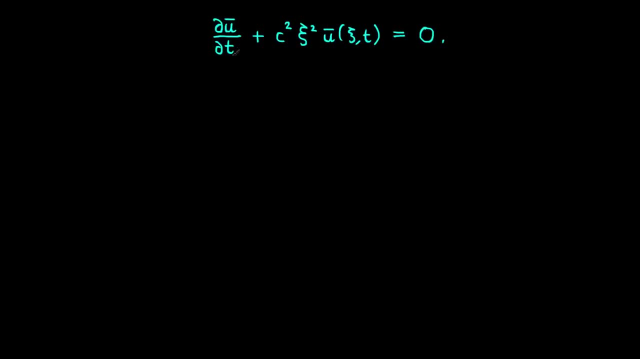 xi and t, but we only have differentiation with respect to one of them, so it's like an ODE. but wherever we would have a constant, an arbitrary constant, in any method that we apply to this from ODEs, we should replace that with a arbitrary function of another variable. so that's going to. 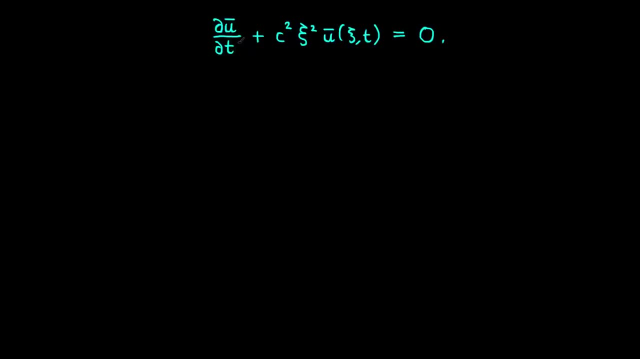 be an arbitrary function of xi in this case. So if we look at this, it's first order and it's linear. that suggests that an integrating factor method might be a good idea. so let's do that. let's have a look at an integrating factor. we choose e to the integral of whatever's in front of the non-differentiated unknown quantity. 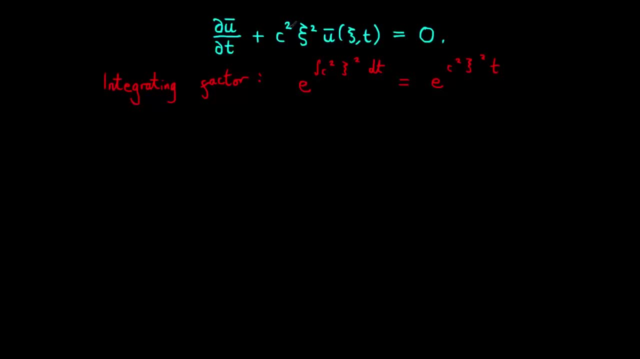 so we'd have e to the integral of c squared, xi squared with respect to t, or in other words, just e to the c squared, xi squared t. so we multiply absolutely everything by that that gives us this expression here, and then you notice that these two terms in fact give us a perfect derivative. 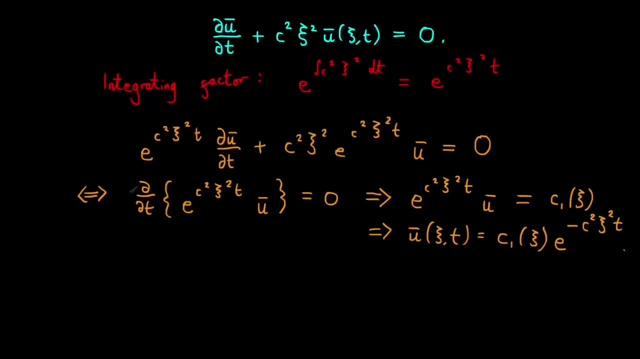 so if you need convincing of that, then you could work in the other direction and you could say: what would I do if I was asked to differentiate with respect to t, the thing in the curly brackets here. Well, hopefully you just got the answer to that question. 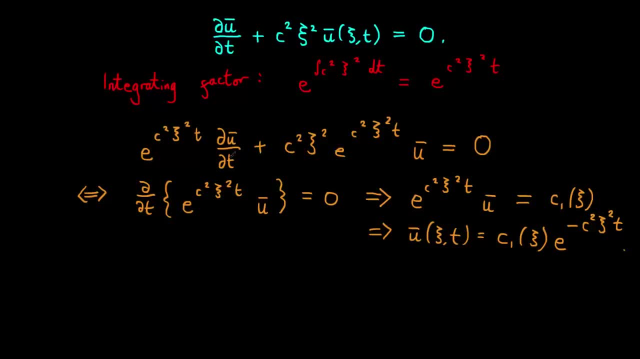 You could use the product rule, so you have the exponential times, du by du, bar by dt, which is this term here- plus c squared xi squared e, to the c squared xi squared t, which would be the derivative of this exponential with respect to t multiplied by u bar. okay, so this is a perfect derivative. 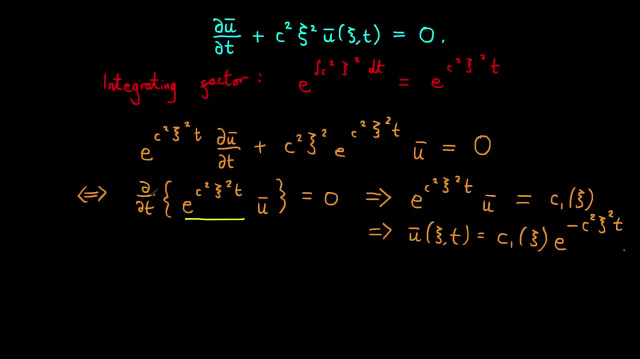 if we integrate both sides of this, then integrating with respect to t of the left hand side leaves us just with the thing from the curly brackets on the right hand side. we'd have a constant normally if it was an ode, but because it's a pde, that is a, an arbitrary function. let's call it c1 of the other variable. 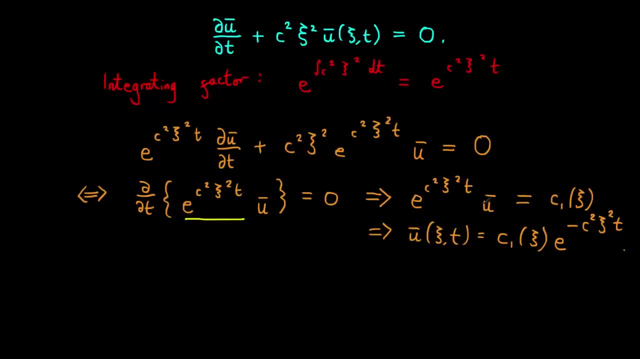 xi. then if we rearrange this, we have that u bar of xi and t is equal to c1 of xi times e, to the minus c squared xi squared t. so now we've got an expression for the transform of u, an expression for u bar, but we've still got this arbitrary function, c1. 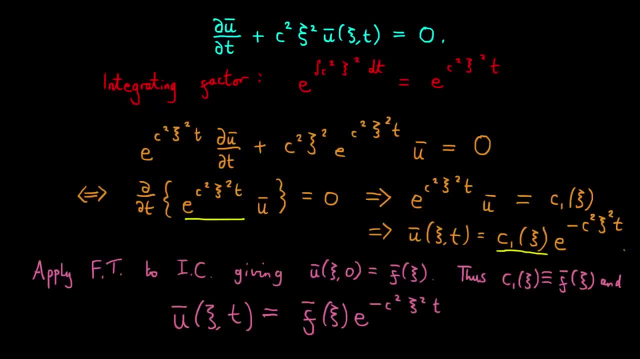 of xi. So to find out what that is, we're going to have to apply the initial conditions. But first of all we have to apply Fourier transforms to the initial conditions. So remember, our initial conditions were that u of x and 0 was equal to f of x. So if we take Fourier, 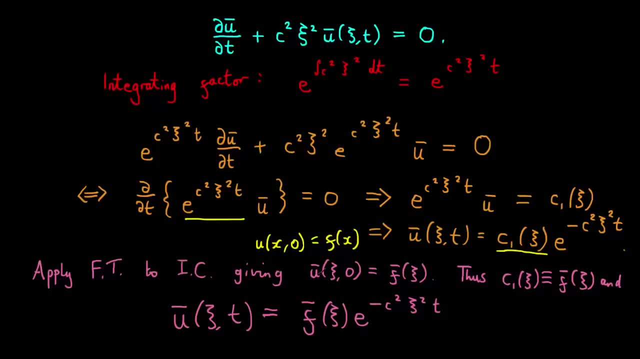 transforms with respect to x of both sides of that, then we'll get u bar xi of 0 on the left hand side, and taking the Fourier transform of f of x gives us f bar xi. And so therefore we can see that if we put t equals 0 into our general expression up here, then if we put 0 here, 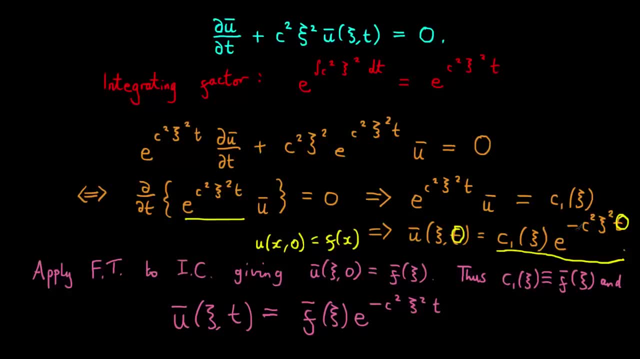 what do we get? Well, we'll have e to the minus 0 gives us 1, so this factor is just 1, and so u bar xi and 0 is equal to c1 of xi, which our initial condition gives us is just f bar of xi. So c1 of xi is exactly f bar of xi. 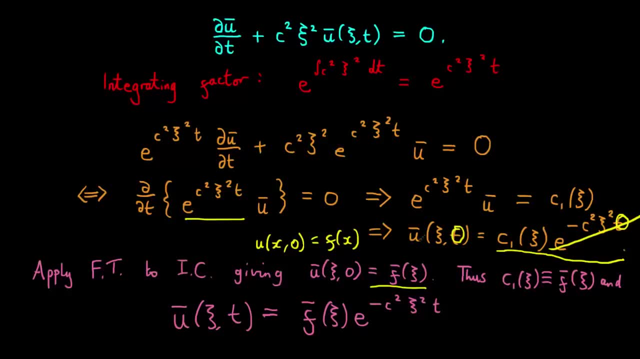 and therefore putting that into the general expression we found in the last step. we have that u bar of xi and t is equal to f bar of xi times u bar of xi e to the minus c squared xi squared t. So that's the first step of our plan that we 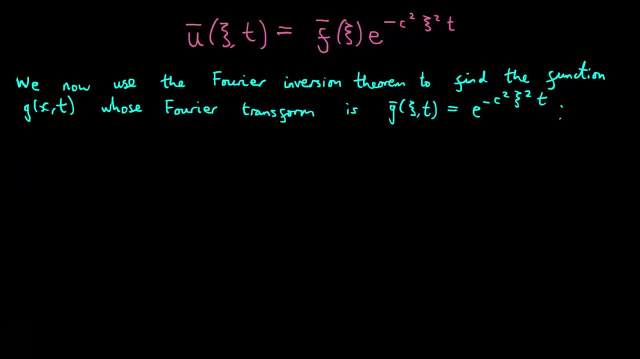 detailed on the strategy part of the video done. So now we progress to the second bit, which is to say, can we find the inverse Fourier transform of the function e to the minus c squared xi squared t? So in order to do that, we're going to use the Fourier inversion theorem. 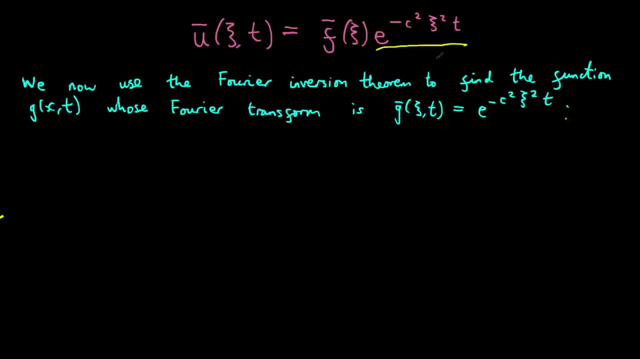 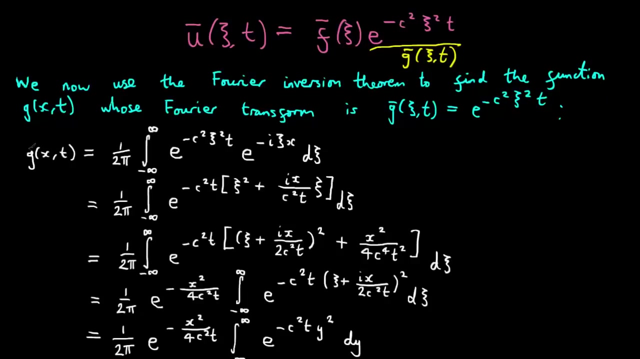 to find the function that we call g, whose Fourier transform is this function that we've called g, bar of xi and t. This is going to be a process that has quite a few steps, but each of the steps are fairly simple. So, first of all, this first line is just a statement. 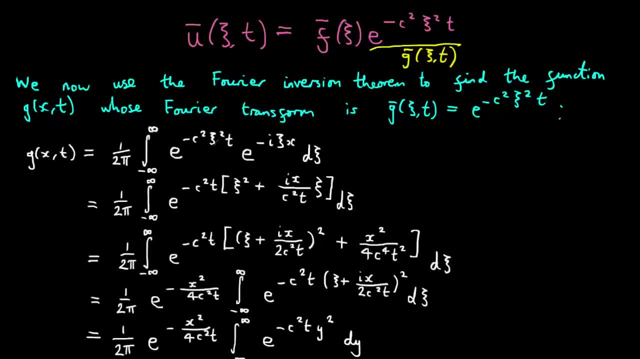 of the Fourier inversion theorem. So it just says that in order to invert the function e to the minus c squared xi squared t, which is what we call g bar, all we do is we take one over two, pi times the integral of that multiplied by e, to the minus i, xi, x with respect to xi. Then, to get to this second line, all. 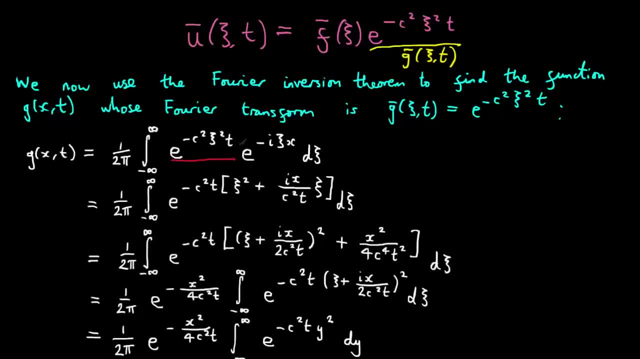 I've done is combine these two exponentials and then in the exponent I factorised by taking out a common factor of minus c squared t. Now that might seem a bit artificial because you introduced this fraction, but the reason we do that is so that the leading term in the square brackets is going to be just xi squared. So this first. 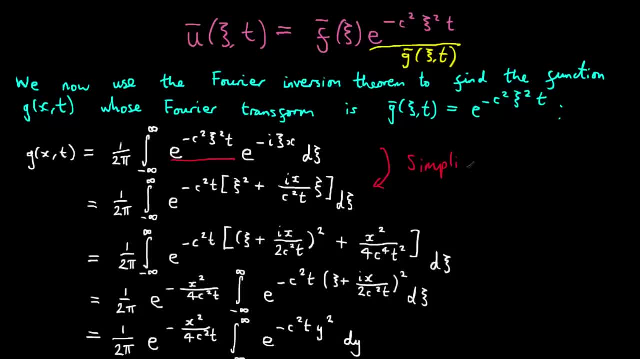 step is really just simplifying. The next step is going to be to complete the square in the exponent. So we're going to write this as: xi plus i, x over two c squared, t all squared. If you think about multiplying that out, we would get xi squared. 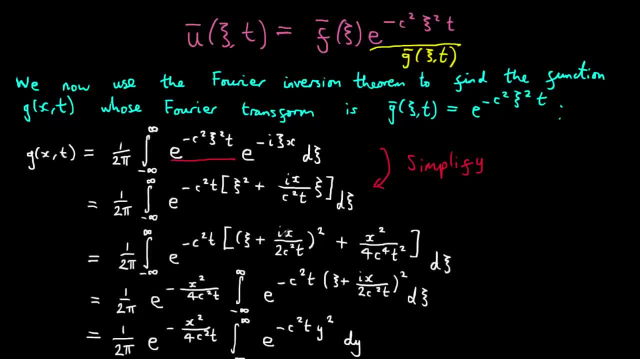 plus two lots of i, x over two c squared, t xi, which would give us exactly this term. So these two terms result. But then we'll have a third term, which will be this fraction here squared. And this fraction here squared would be i squared, which is minus one times. 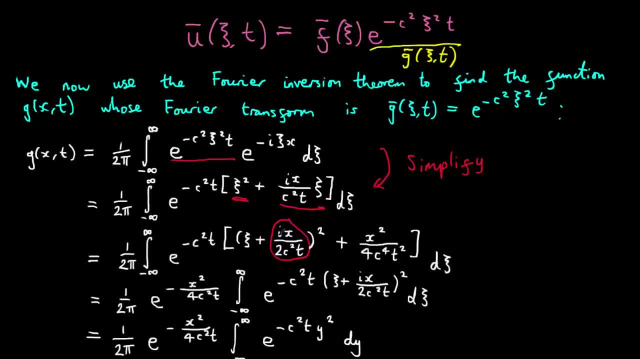 x squared over the bottom squared, So we'd have minus x squared over four c to the four t squared. So consequently we have to add that term back on. So we add on x squared over four c to the four t squared. So this step here to get from the second. 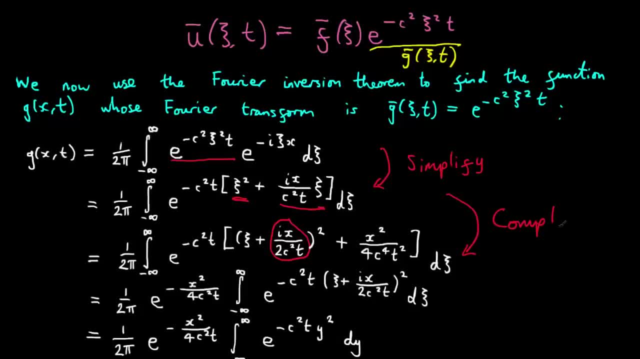 line to the third line. we're just completing the square. Now what about the next line? Well, we can see that this last term is going to give us an e to the minus c squared, t x squared over four c to the four t squared. There isn't a xi anywhere. 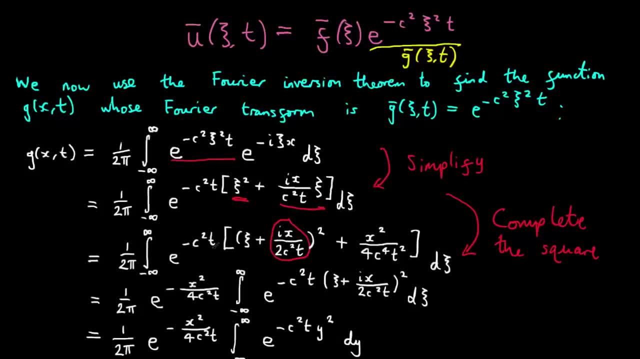 there, which is what we're integrating with respect to. So we can take that exponential outside the integral And that leaves us with one over two pi, e to the minus x squared over four c squared, t times the integral of e to the minus c squared t, multiplied by this. 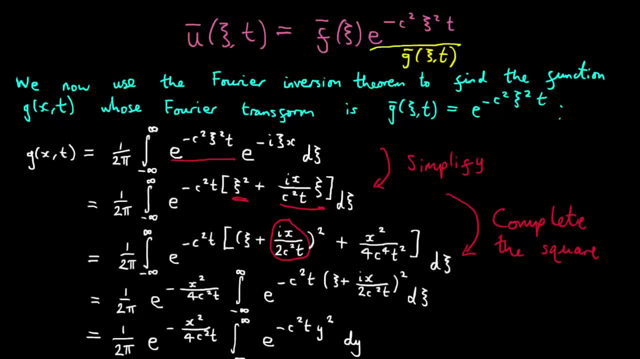 bracket that we've got squared with respect to xi. The next step's going to involve a couple of substitutions. So the first substitution that we're going to do is to look at this bracket here and call that. let's say y, So y is going to be xi plus i, x over two, c squared t. Okay, that means that dy is exactly. 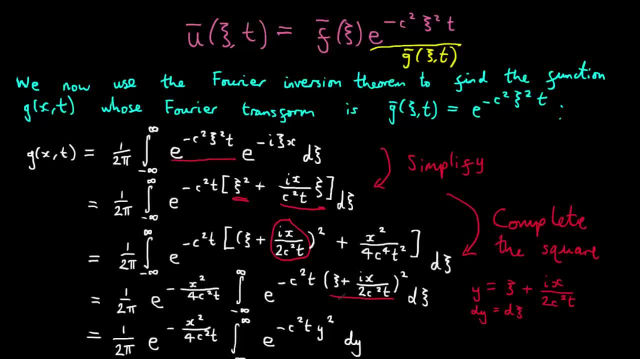 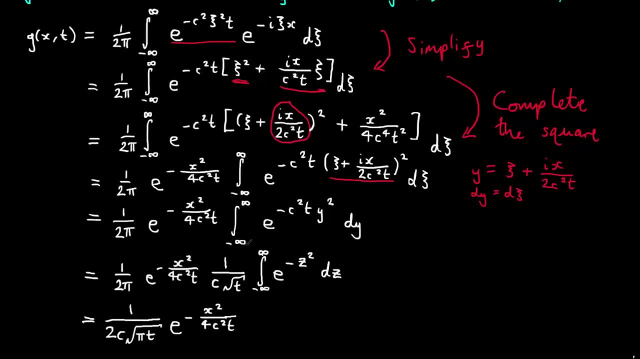 d, xi, And so if we make that substitution we are going to get this expression here. So the integral becomes the integral from minus infinity to infinity, e to the minus c squared t, and then we have the bracket squared. before now we've got y squared. 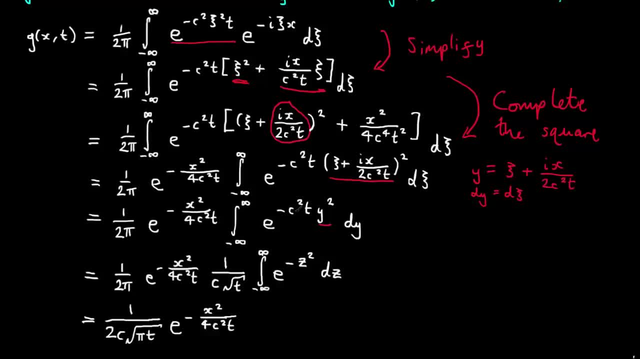 The next step is going to be to make the whole exponent equal to minus z squared. So to do we're going to make the substitution that z is equal to c squared. well, in fact, z squared will be equal to c squared, t y squared. In other words, we're going to define z to be the square root of. 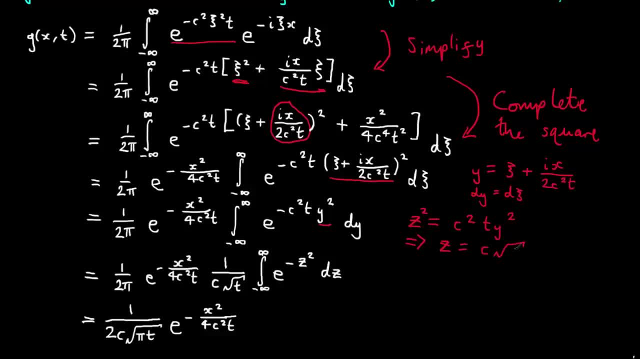 this. so z is going to be c times the square root of t times y. In other words, dz is going to be equal to c root t dy. Okay, so when we write dy well, dy will be dz over c root t when we make. 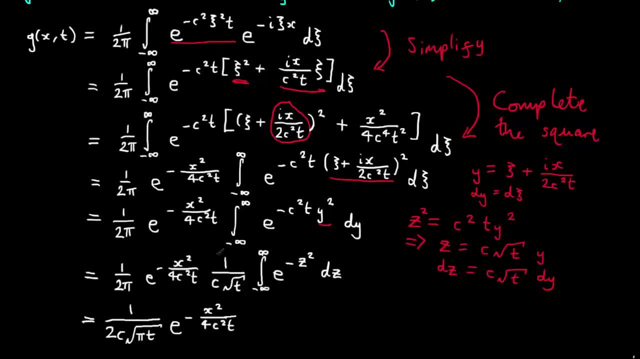 the substitution. so we're going to have a factor of 1 over c times the square root of t coming in. but then the integral, finally, is going to be a nice one, because we're going to have the integral from minus infinity to infinity, of e to the minus z, squared dz. 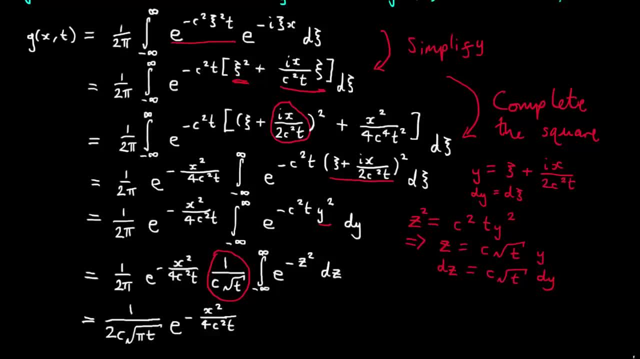 And this is a well-known integral and although we haven't proved it in the course, you'd always be given this result- then this integral is equal to the square root of pi, and so this whole integral simplifies really nicely just to the square root of pi. Therefore, putting that into here and 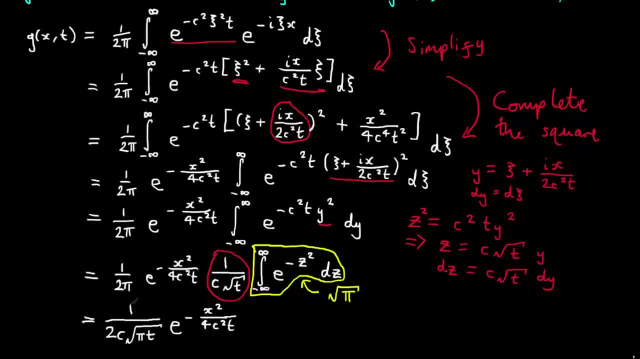 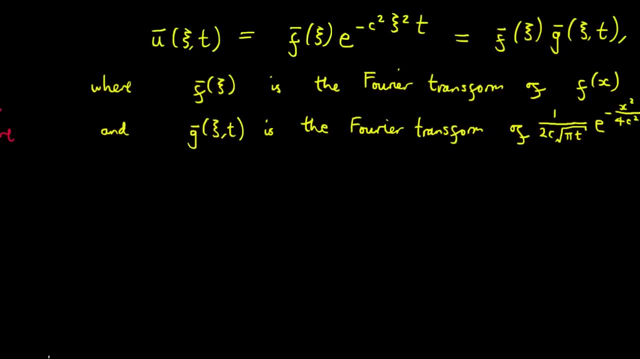 simplifying, we get that g of x and t after all of those steps is equal to 1 over c squared t over 2c, root pi t e to the minus x squared over 4 c squared t. Finally, let's collect together the results that we've got so far and use them to finish. 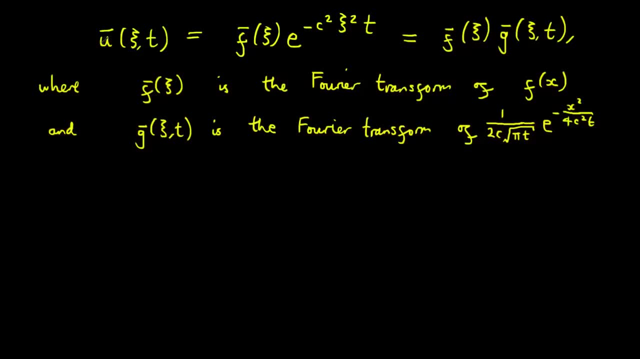 the problem. We've said that the Fourier transform of u can be written as the product of Fourier transforms. It's the product of f bar and g bar, and we further know what the inverse Fourier transforms of both those functions are, because we know that the inverse Fourier transform of f bar is just the function f of x, and we also know that g bar of xi and t is the Fourier transform of the function that we've just found. 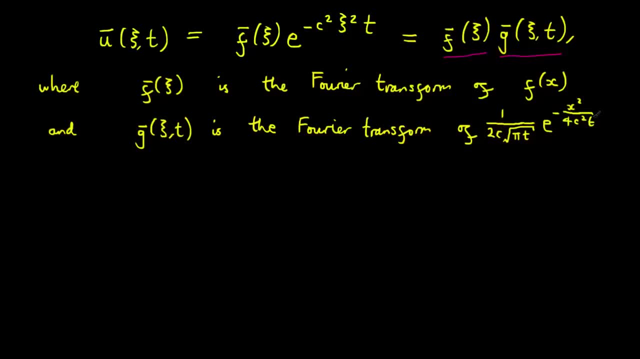 So 1 over 2c root pi t e to the minus x squared over 4 c squared t. So because we know that the Fourier transform of u is the product of two Fourier transforms, we can use the convolution theorem to tell us that the 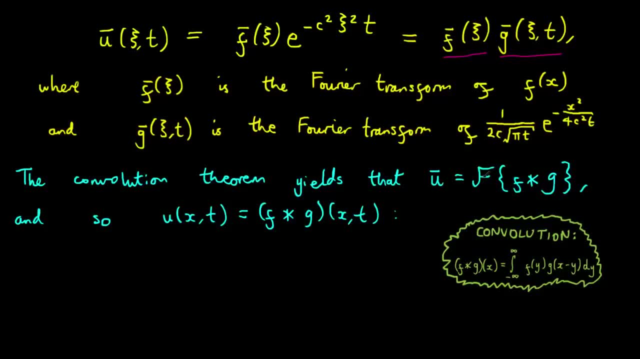 product of the Fourier transforms is exactly the same as the Fourier transform of the convolution. Remember, this is the definition of the convolution in green here. And then, finally, if we apply inverse Fourier transforms to both sides of this equation here, then the inverse Fourier transform of u bar will just be u, so that will be u of x and t. 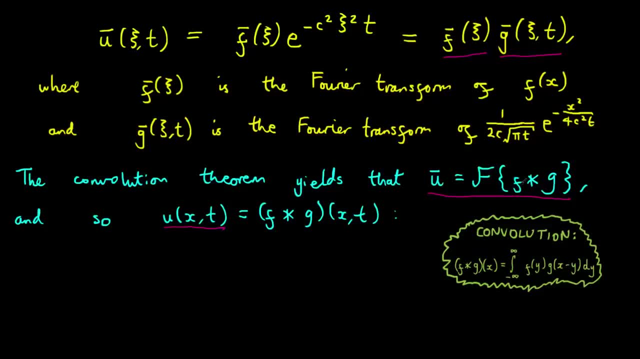 and then the inverse Fourier transform of the Fourier transform of the convolution. Well, those will just cancel each other out: the inverse Fourier transform and the Fourier transform. So we'll just have the convolution of f and g. Okay, so u will be the convolution of f and g. Here's the definition of convolution. 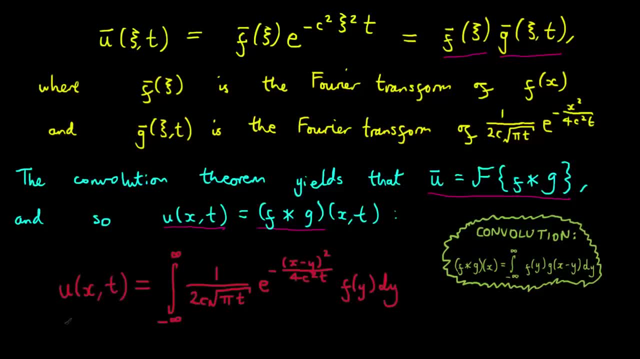 All we need to do is apply that to f and g and finally we get the result that u of x and t is the integral of 1 over 2c root pi t times e to the minus x minus y squared. this is g of x minus y over 4c squared t multiplied by f of y. 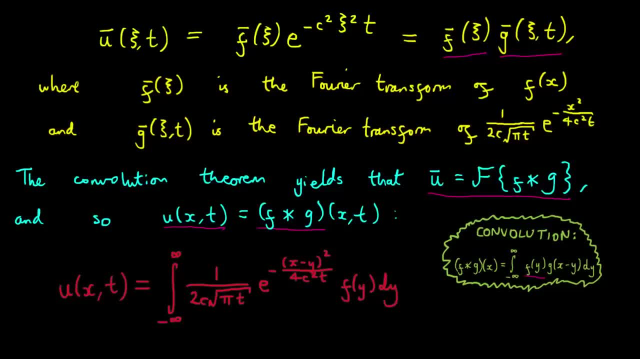 and integrated with respect to y, And that completes the solution to the heat equation Cauchy problem.